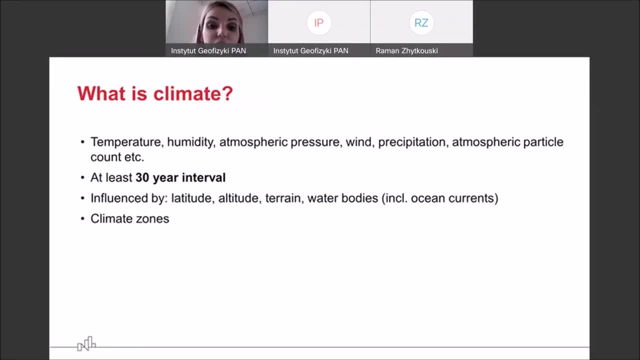 humidity, atmospheric pressure, wind, precipitation, but also atmospheric particle count. So these are the conditions that we may observe, but the conditions that we observe on a daily basis are actually weather and not climate, Because the crucial difference lies in the time interval. 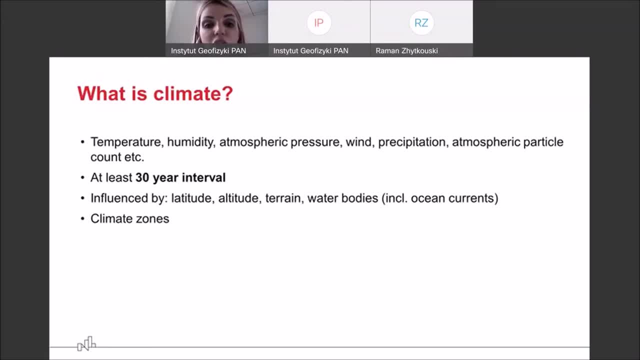 So to talk about climate, we need a longer measurement series, a lot of data, And the conditions that we compare are conditions from, we tend to say, 30 years period at least, And the climate is influenced by many factors. This is why it's we don't have the same climate on the whole planet. 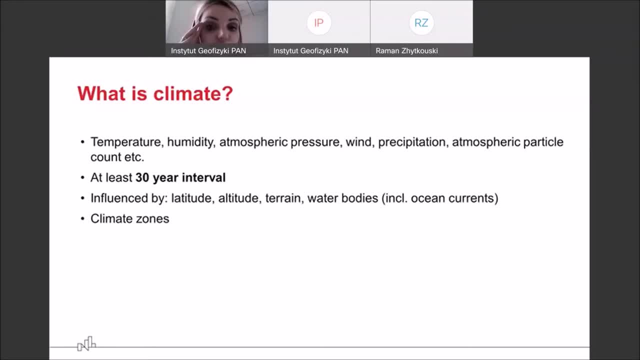 So we have the influence of latitude, altitude, also terrain, landscape, large water body, water bodies like especially large water bodies such as seas or oceans, but also smaller water bodies have some influence as well, If we talk about oceans. 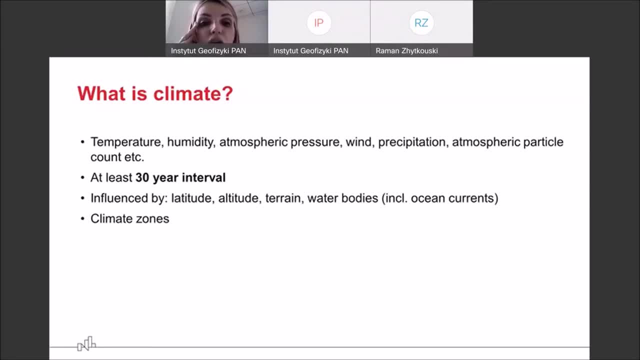 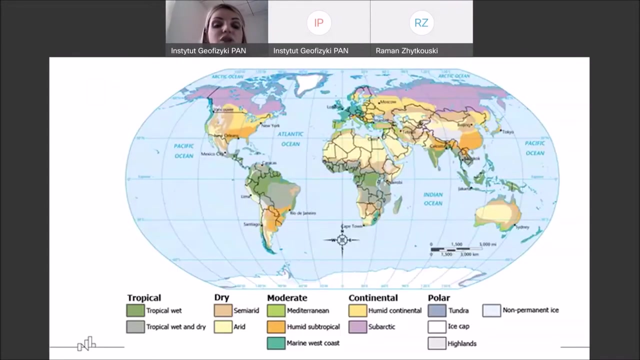 We need to remember that ocean currents have a very strong influence on climate as well, So the fact that climate conditions are different in different parts of the world. because of those factors, we have so-called climate zones. That means we describe climate using climate zones. 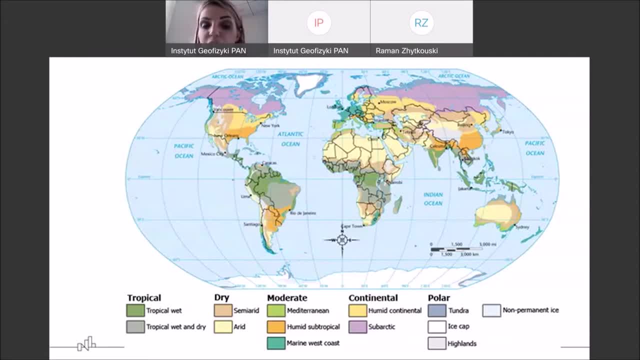 And we- we we're doing so- had been doing so for a very, very long time, starting from antiquity. So people tend to categorize things and search for similar features, And this is how climate zones are compared and described. So there are a lot of classifications we have. 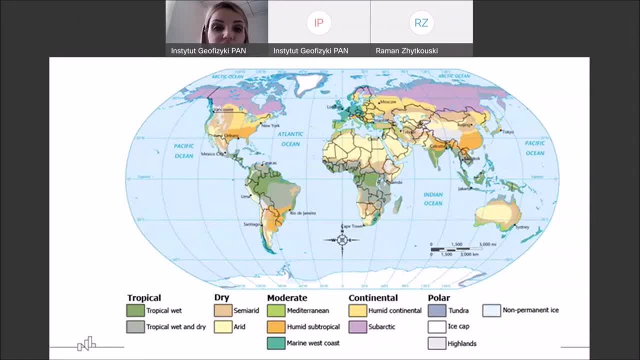 And and and they are somewhat different, but in general they're they're also quite similar. We also we always have polar zones With ice caps. we also have content to the climate. We have tropical climate, dry and moderate, and the difference is mostly in in details. 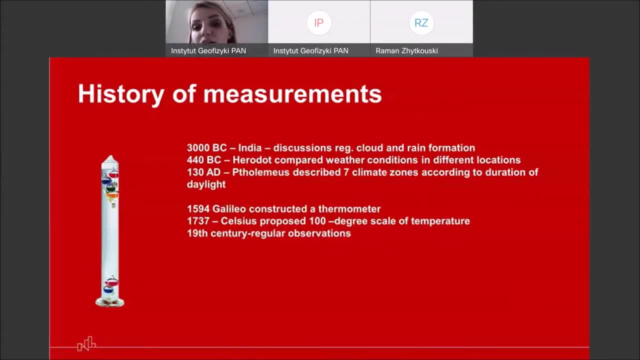 So, um, When I talk about climate, I wanted to emphasize that The time interval Interval is crucial here. so the 30 years Time- that is period, is crucial. So, uh, it means we need a lot of measurements and we constant and uh measurements and we do those measurements reliable. 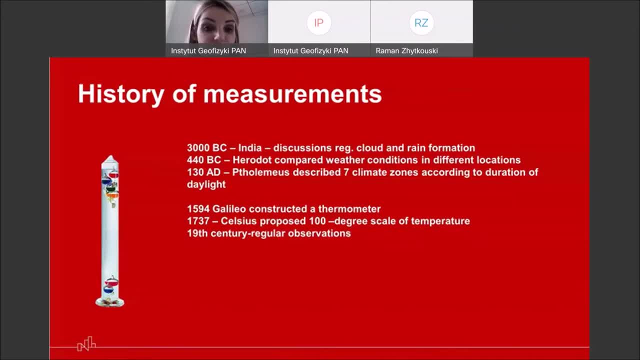 Results, reliable data that are delivered on regular basis. Uh so, uh Yeah, Just like with describing climate zones, and you can see, uh, the 1st, 1st and known To try to describe climate zones. so we were in very early in our history and he was basing his 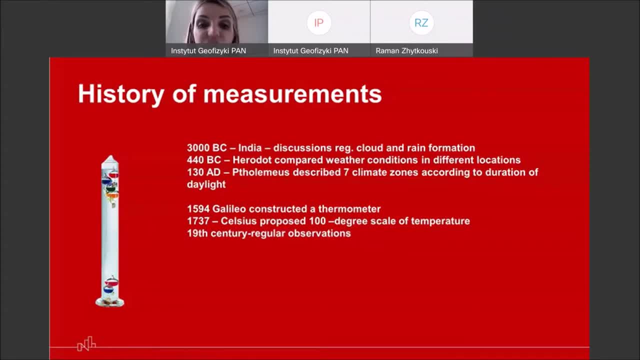 His classification into 7 climate zones on duration of daylight, which is also 1 of the factors that Is crucial for climate conditions. Uh, but uh, even, Even much, much earlier, like 3000 years, or price. 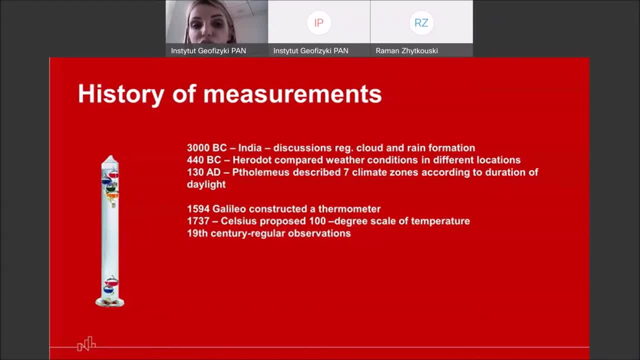 Uh, people were already discussing Climate conditions, that just they were Trying to figure out how Our clouds, or why does it rain, Why does Rain sometimes, and sometimes it doesn't know, sometimes it's dry, And But there were no actual measurements and of course, we have no. 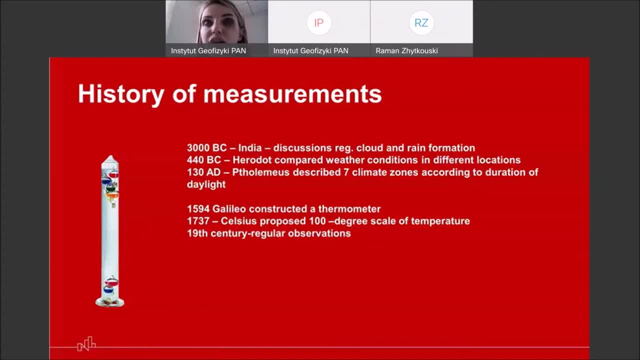 Reliable data in the sense that we have Data, we collect data now, from this, this period, Uh then, with more and more instruments and more technology, we gained access to, To new data, to large data sets, to data from large- Uh large- parts of of the year. 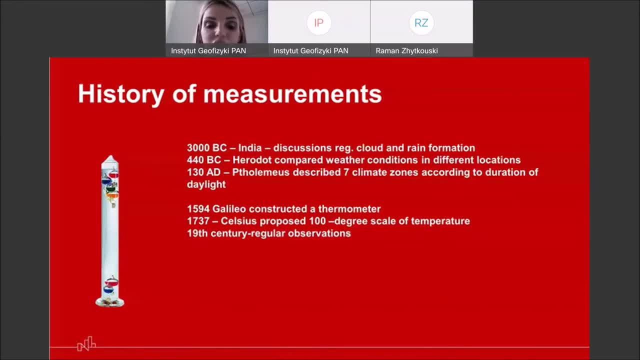 And the database. Uh, it's constantly growing, So, but we started really simple with with a thermometer. what you can see here on the left Is a thermometer constructed by Galileo At the end of 16th century. now it's more like a decor. 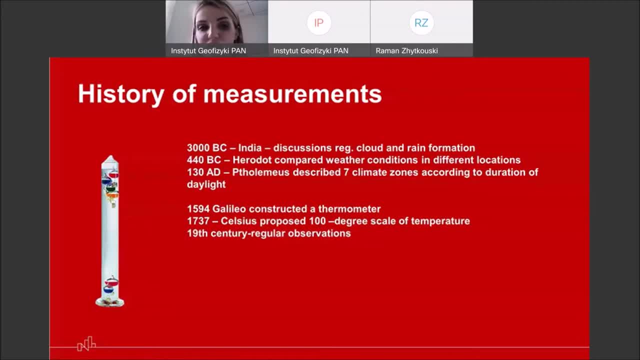 Uh, Uh. it used to be very popular, uh, as a, As a tech item, uh, but it really worked. So we had something to measure with. Uh, then another Crucial date in history of measurements. We measure things, we measure temperature, but what is the scale that? what is the? 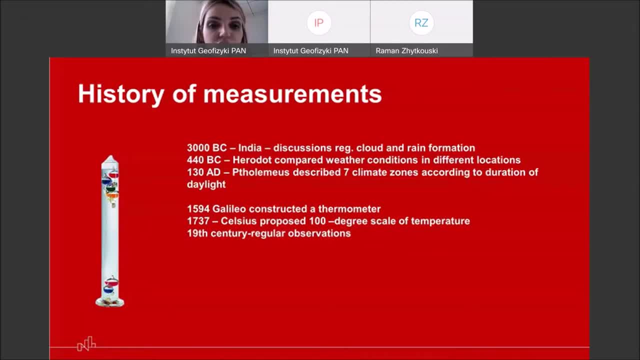 Common scale that we are able to use. there are many scales, but 1 of them, and 1 of the most widely used, is Celsius Uh scale temperature, which has 100. Uh degrees, So 100 degree scale. 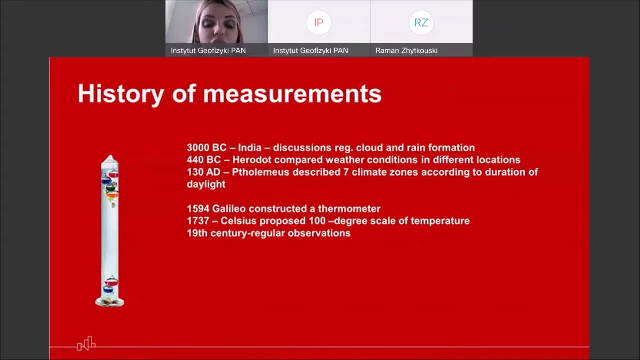 In 19th century, uh, we, We began regular observation. We began regular observations With new technologies such as electricity, such as telegraph, Uh, we gained access to Rapid exchange of data, rapid exchange of information. Therefore, 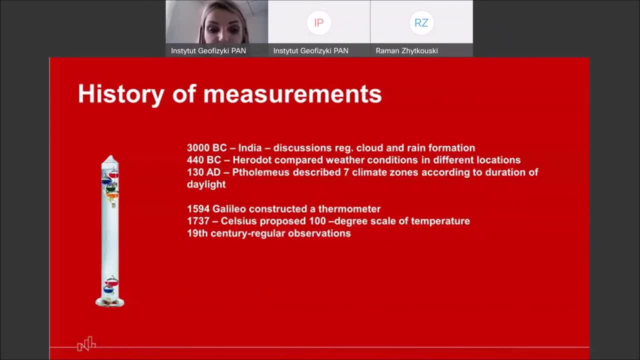 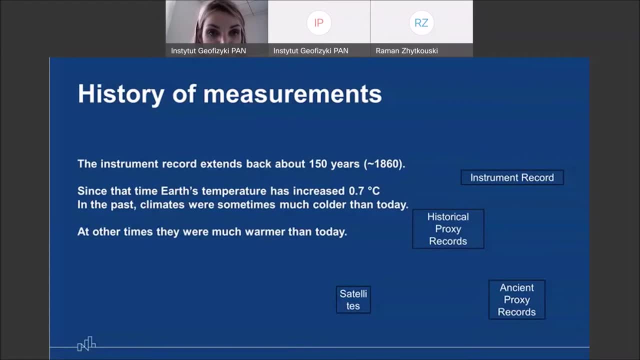 Uh, we could measure more and be more efficient in our uh. so The, the instrument record Extends back about 150.. 50 years. So So second half of 19th century we started regular measurements and it's so-called the longest data set. 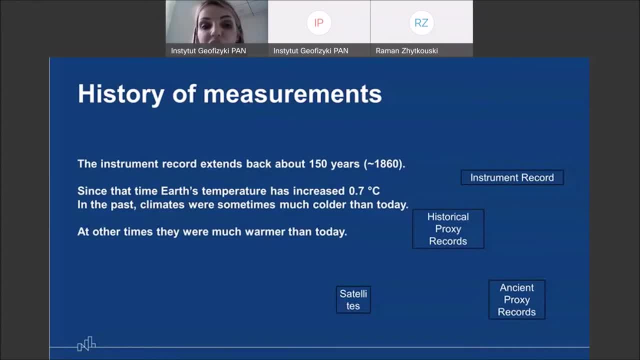 Of course now we have satellites, we have very modern equipment we have access to. we can exchange data and store data and work with data and model it and combine it, combine the data sets, databases, very fast and very efficiently. So we know that since that time, since the start of regular measurements, we have a lot of data set. 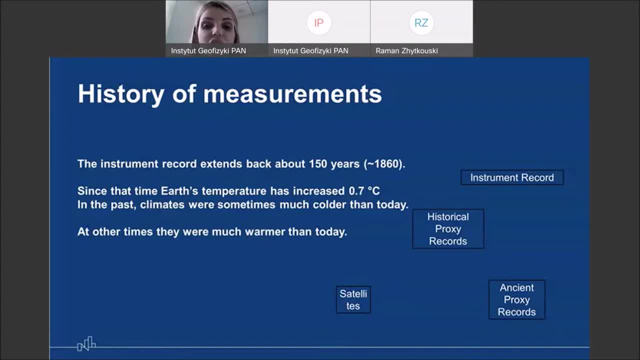 So we know that since that time, since the start of regular measurements, the Earth's temperature has increased about a little less than 1,000 degrees compared with the second half of 19th century. So we also know that in the past climates were sometimes much colder than today, but other times they were also much, much warmer. 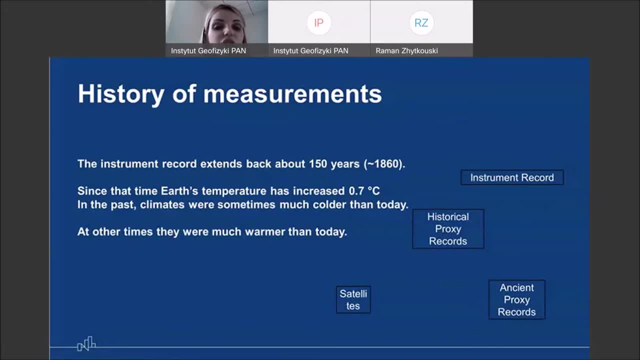 Now, how do we know that? Because now I'm referring not only to the time- There are time periods that are much earlier, much far away on a time scale, far back on a time scale than the beginning of regular measurements in the 19th century. 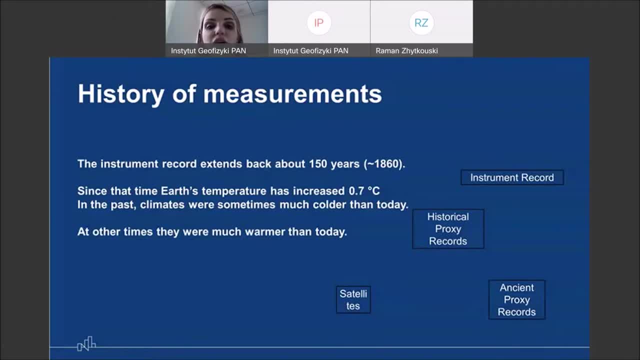 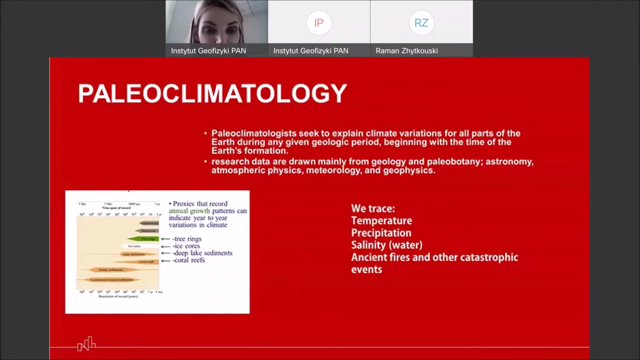 So here's what, where we go actually to our main topic, which is paleoclimatology, and some terms that should be associated with paleoclimatology are historical proxy records and ancient proxy records, proxy records in general. So what do paleoclimatologists- wrong word- do they seek to explain or research what the climate looked like in the past, before the measurements were even possible, before even humans were present on Earth? 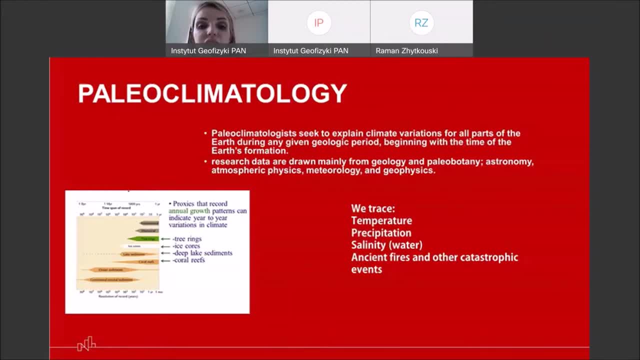 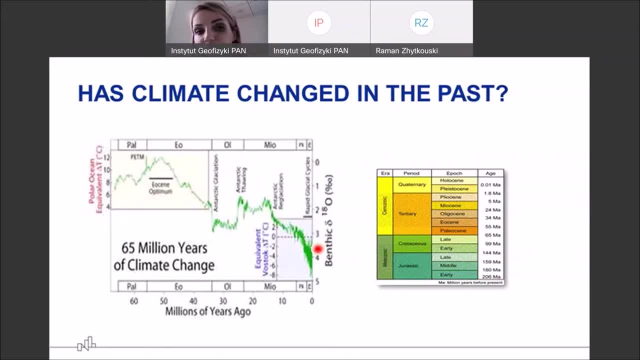 to our past climate conditions, uh, but we have to be aware that those conditions were not, would not have been, supportive to our light. we wouldn't be able to live in such conditions when, for example, dinosaurs were on earth. not just because of dinosaurs, because of many other things and many other things related to temperature, such as 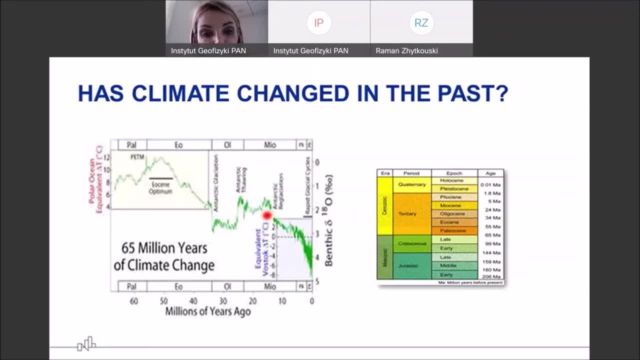 ocean levels, for example, and at some point, uh, ice caps, large ice sheets appeared. first the antarctic ice sheet, then greenland ice- inland ice in in greenland, and that means that a lot of water got trapped in in the ice. so that means that the ocean levels dropped significantly at that point. 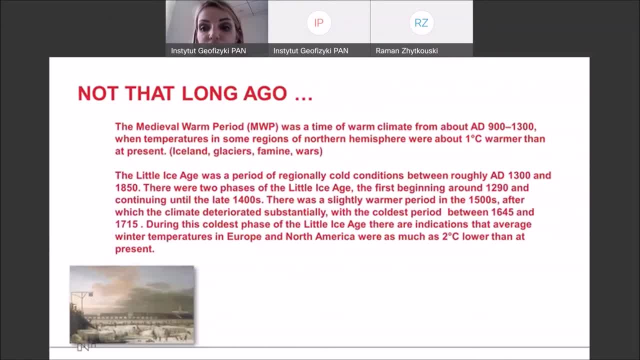 uh. so i went back to, uh, uh, i went back to, like time of dinosaurs, 65 million years ago. but um, there are also some branches, some domains in our climatology that are much closer to uh, to us. it's so called um historical, um climatology, let's say so. so um, or environmental history, so environmental history. 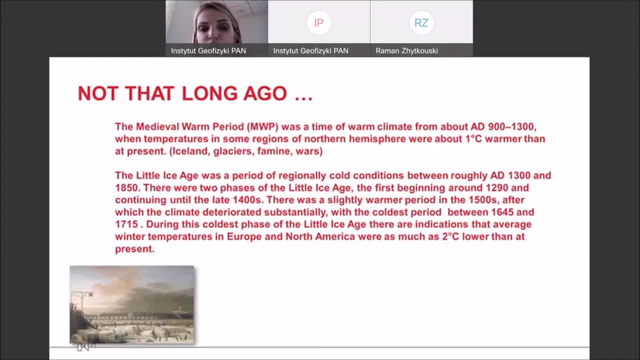 is a rather new discipline. uh, it was more like the 1960s, 1970. uh, so it was like a consequence of the growing awareness of environmental problems such as pollution, air pollution, water pollution, um, depletion of ozone layer, which is a huge issue at the time, uh, enhanced greenhouse effects and so on. so people were interested what it looked like. 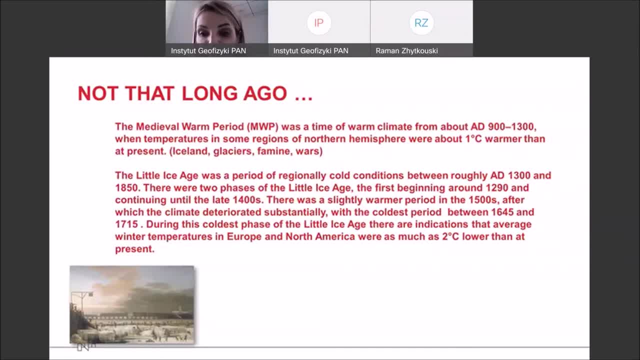 in the past to compare with how we affect earth. historians- not climatologists, but historians- started to look for the origins of the contemporary problems, And they were using many different sources like paintings, autographs, some recorded observations, books and so on. So historical documents contain a lot of information. 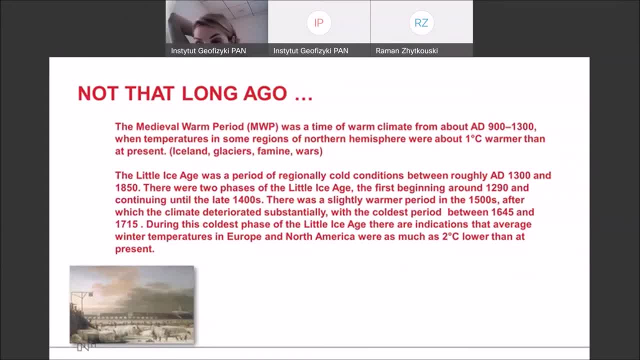 about climate but also description of the landscape at some point, And it was all used to reconstruct climate and landscape change dating back several hundred years in time. So you can see that we there were two very significant periods identified, three, maybe because one of them can be divided. 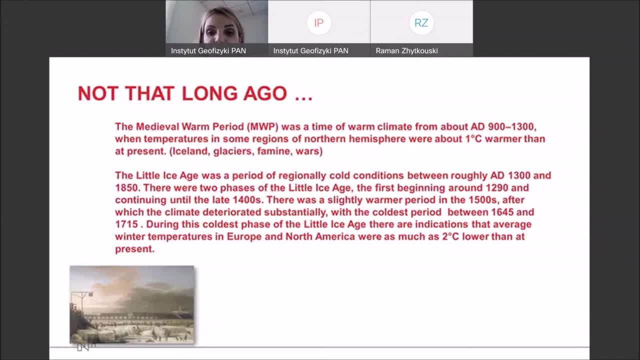 into two periods at least, But I can say that with properly evaluated historical data can give us lots of quantitative and qualitative information about climate, And thanks to that, we identified two periods That were not measured directly or where there were no direct measurements yet, But still. 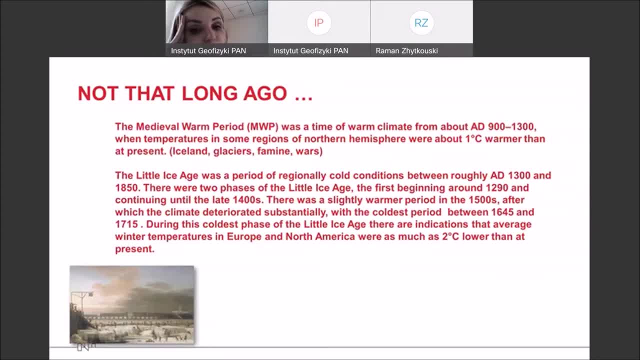 we have some information that confirms what the climate conditions were like. First one is so-called Medieval Warm Period, MWP. It was a time of a warm climate- warmer climate, at least in Northern Hemisphere- which dates about 19th century. 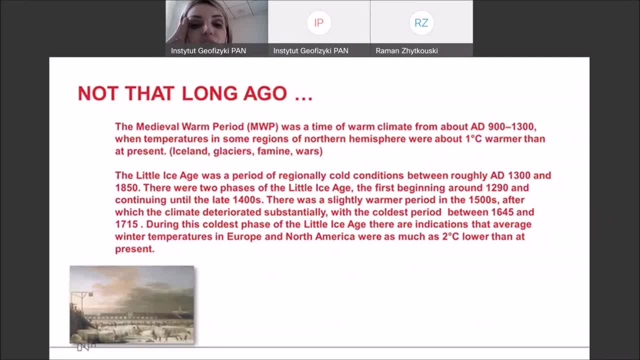 19th century. 19th century And the year 900 to 1300.. So the temperatures in some regions of Northern Hemisphere were like one Celsius degree warmer than at present. Then there was so-called Little Ice Age, And then the conditions were very cold, at least in some regions of ice, And it started after. 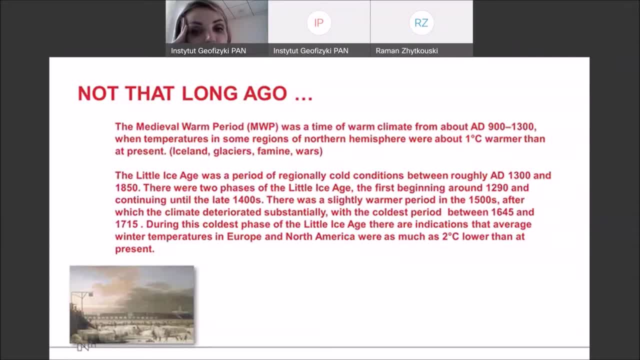 the medieval warm period And it's roughly 14th century up to half of 19th century. So there were two phases, like I said, of Little Ice Age And in general the coldest period was between 19th- sorry- 1645 and 1750.. 1750. 1750. 1750. So it is coldest phase of Little Ice Age. The winter temperatures in Europe- and now Samaritania, because that's where we get most records from- were even two Celsius degrees colder, lower that is, And this period is related to lots of agricultural. 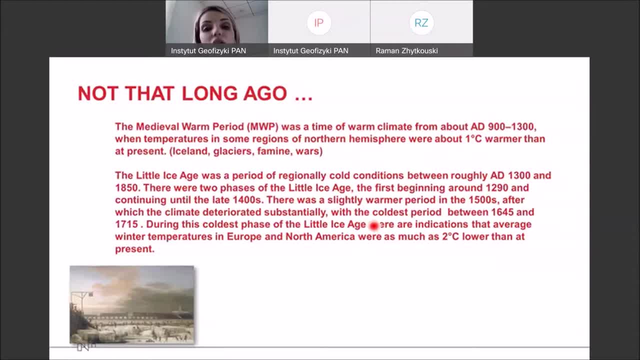 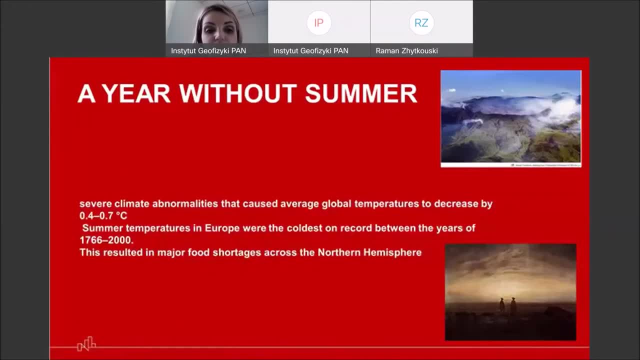 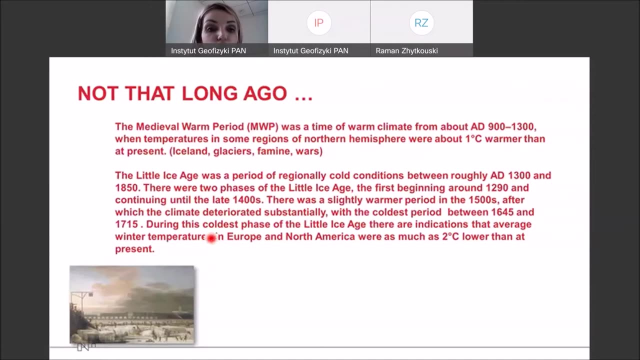 problems: problems with crops And, as a result, lots of famine with agriculture, a lot of problems with forests, Right Correct, in lots of wars. they were not good times in general. So I mentioned paintings, and this is one of those paintings that we can draw records from. We don't have direct measurements, but we 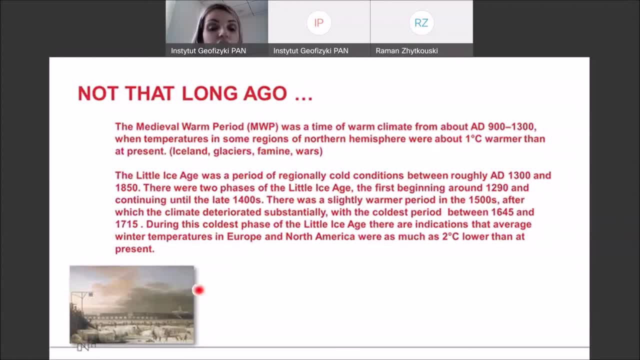 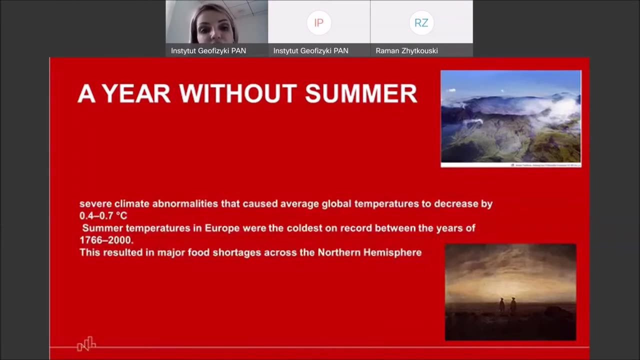 can see the Thames, the river Thames. it's a very large river, completely frozen at some point in 17th century, So it means it had to be significantly colder than now. One more thing that is also related to environmental history and past climate. 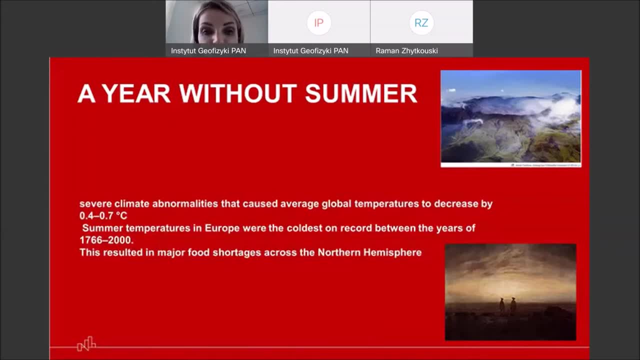 conditions, A very famous year without summer. The year without summer is the year maybe some of you know When was it, This very peculiar 19th century disaster? It took place in 1860 and in 1860 the weather in Europe and North America took a very bizarre turn. 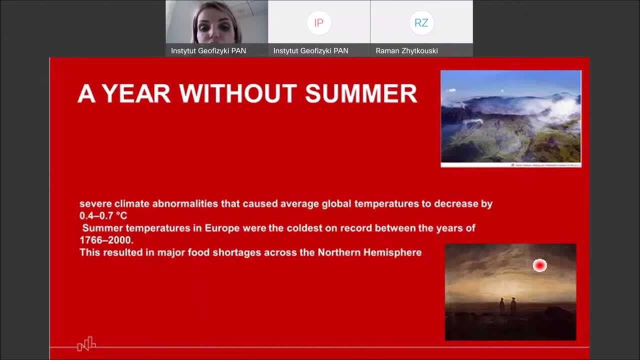 and that resulted in very widespread crop failures and, in general, I would say, feeling of apocalypse. So the weather in 1816 was really unprecedented, at least from the point of view of people who lived there, And so spring arrived as usual, but then it seemed like seasons started to turn backward. 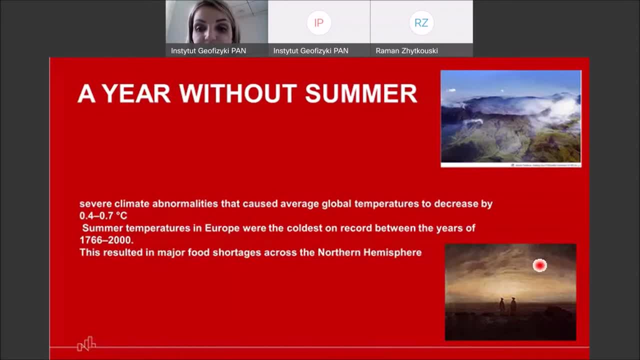 So the cold temperatures returned. In some places the sky appeared like permanently over, So there was a lack of sunlight. It became so severe that farmers lost their crops. There were food shortages reported in Ireland, in France, in Manila, etc. England and the United States. so it had a lot of consequences, also historical or 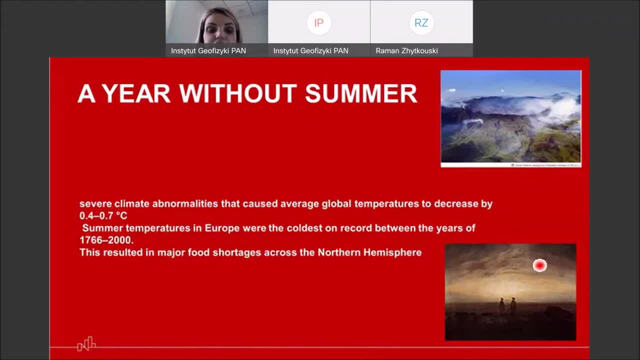 geopolitical consequences. so the famine, especially famine in Ireland, and made people try to look for new places to live, and so it it accelerated the migration rate. so we used to have also climatic refugees. we now predict that climate change will cause a lot of new waves of refugees and there were climate 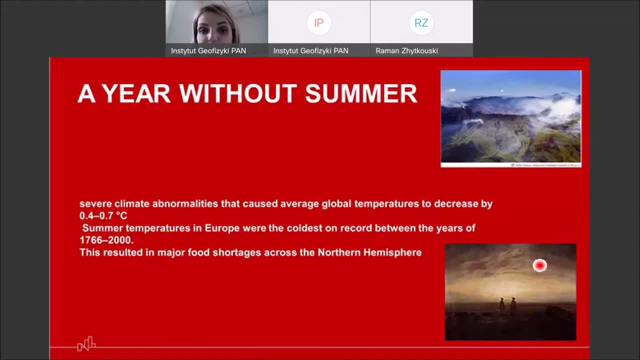 refugees in 19th century and it also left some trace in literature and art. so in Europe, this glue glue me, whether hopeless cold will be, whether help to inspire, for example, the writing of a very, very famous book by Mary Shelley, a classic horror tale, Frankenstein. so it did leave some. 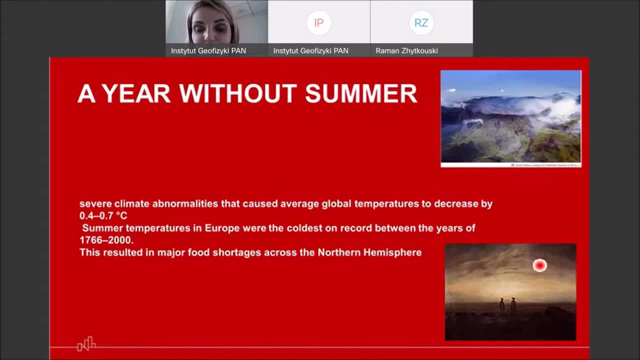 some trace in our culture, so it would be more than a century. so it was created by when a przez Comes came a new generation. Kant happened to Меня and Nor Creator and he comes back from Nor Creator and enters England and hardwired 나와. 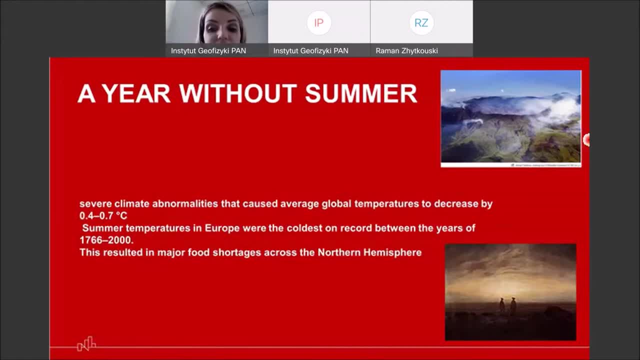 and themselves here, by pasaí No lagoon, into the atmosphere, into the upper atmosphere, and this dust from this volcano. the volcano is called Mount Tambora, it is here. it shrouded the globe, and so the sunlight was almost entirely blocked, and this is why the 1816 did not see a 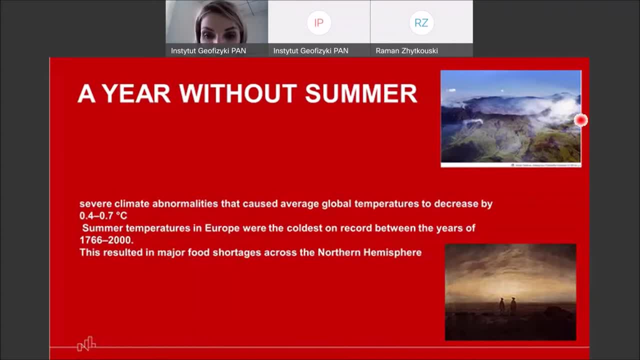 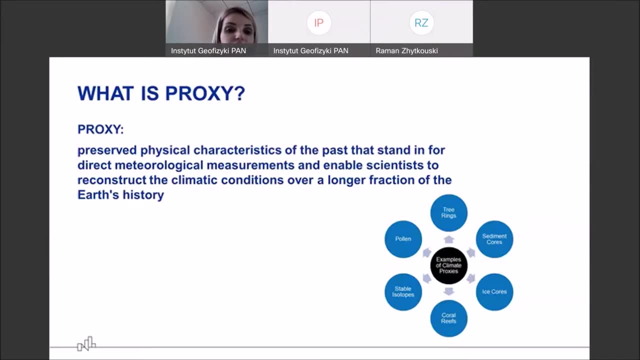 normal summer. So, as you can see, such an event can bring a lot of trouble but also shape our culture and history in very surprising ways. I don't see an app called, As I mentioned several times before. we do not have. we sometimes have direct. 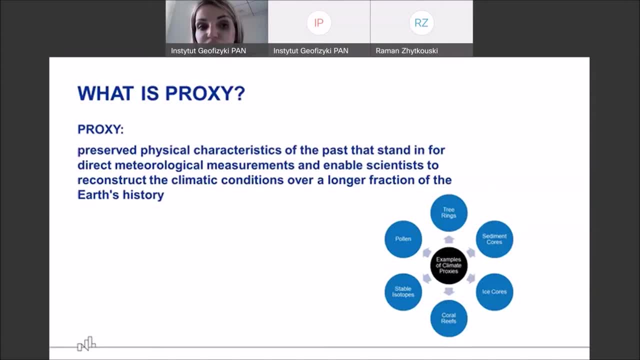 observations in case of a volcano. but we do not have any direct observations in case of a volcano, of environmental history, but in case of climate conditions dating back to 65 million years ago, we don't have observations and we certainly don't have. 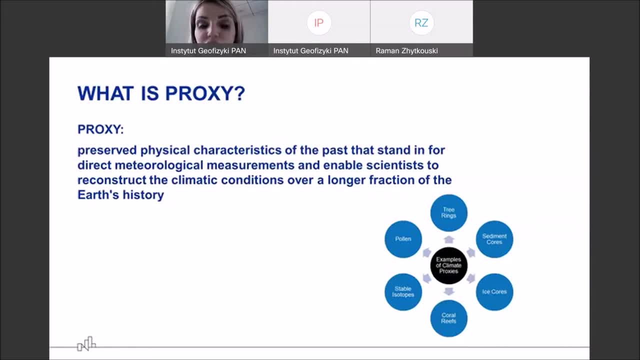 measurements. so we need to use something else, and our climatologists need to use something else, and what they use is so-called proxy Proxies, in general, something that represents something else indirectly, So in some elections, a voter. 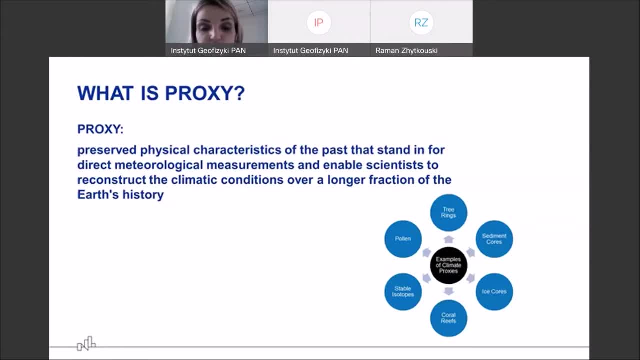 can choose another person to cast the vote, so this other person is a proxy, And there are many, many proxies. that means indirect data for past climate, and they provide a lot of information, but none of it is really perfect and we need. 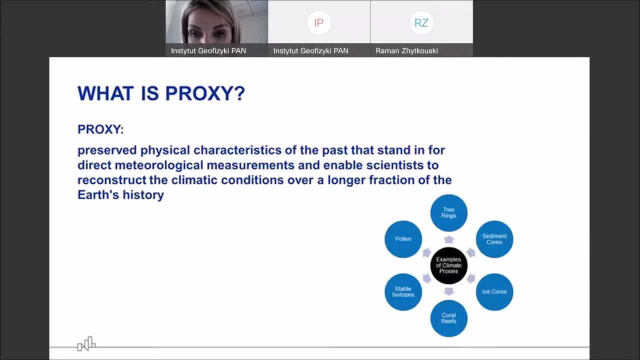 to combine a lot of information to get the whole picture. Some information, like kinds of past plants and animals, are quite easy to understand, and some important proxies involving, like chemical elements, oxygen isotopes, are more difficult to comprehend. But all these examples that you can see here 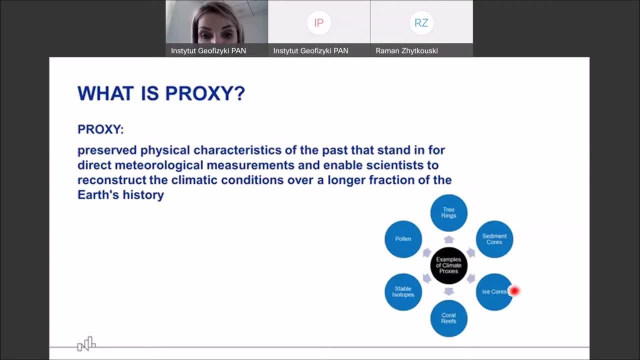 these are the examples of proxies such as isotopes, ice cores or data drawn from ice cores. rather, pollen, tree rings, sediment cores, coral reefs. they are used individually or together. they can help us piece together the past climate of a particular time and time period, and also a particular region. 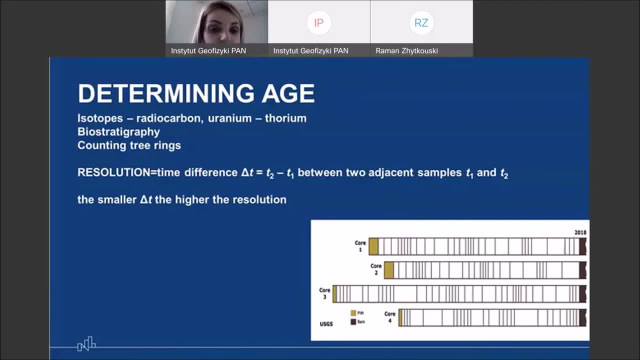 So first we need to determine age. If we have a sample, if we have a proxy, we need to determine its age to find out which period it represents. So there is a variety of analytical techniques. These techniques are used to determine the age of those archives, of those proxies. 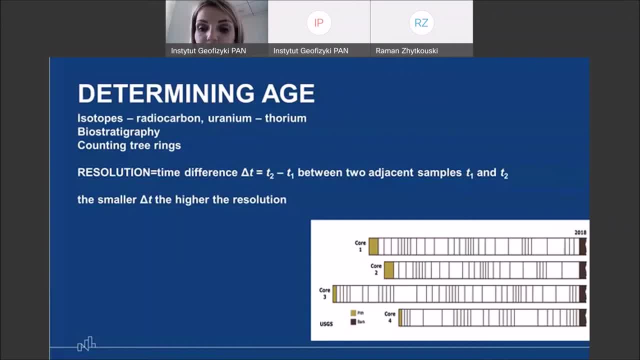 Uh, typically we are using isotopes and its so-called radiocarbon dating, but it dates back not that long ago really. So we analyze the nature of radiocarbon with isotopes such as radiocarbon or uranium thorium, which are present in sample material. 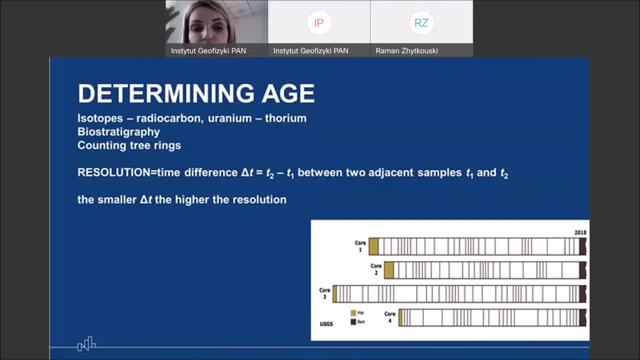 And we can determine so-called biostratigraphy. So we have samples, we have some fossils and we can say which one was earlier appeared earlier, which one appeared later, but also its exact age. There are also other techniques and we can also use rather simple techniques such as counting. 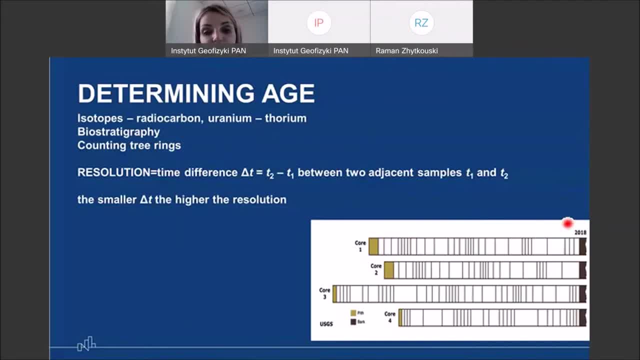 tree rings. If we count tree rings, we can date back from the day, from the year the tree was taken down, back to the time it started to grow, let's say. And another important thing about determining age of proxy and also how exact is the data proxy brings us, is so-called resolution. 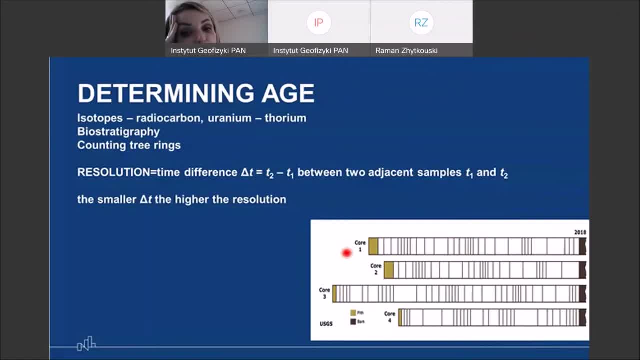 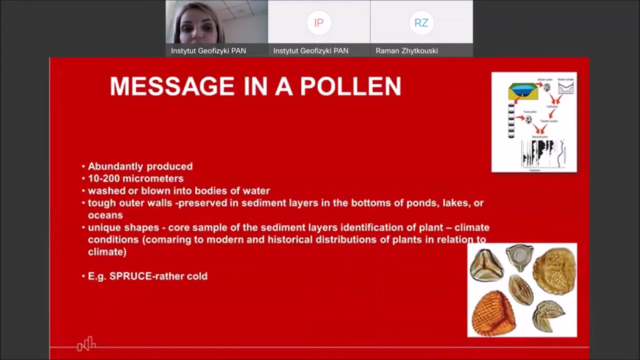 And resolution is as a time difference between two samples. So the shorter this time period is, the more exact data we receive and the resolution is then higher. I mentioned some of the examples, and one of the most interesting, durable, are pollen. The pollen grains are reproductive. 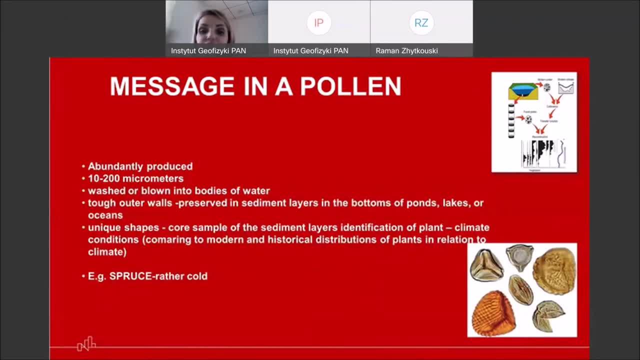 bodies of seed plants and each of these grains has very unique shape depending on what plant it comes from. They are very durable. they are hard to destroy because they are made of substance. they're protective by substance known as propolini, which is very stable, chemically stable, very strong. 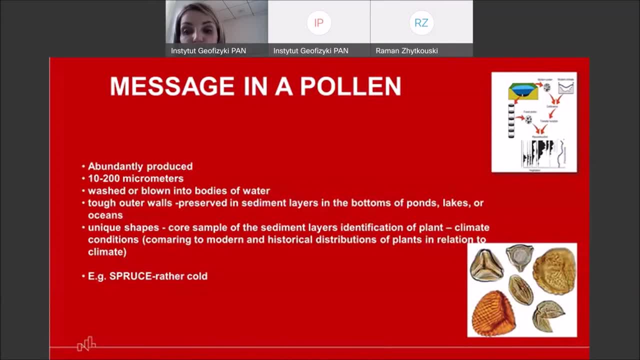 So when these pollen grains are washed or blown into water, into the ocean, can be preserved in the sediment layers in the bottom. So if we draw them from the sediment layers we get those little messages messengers in the bottom. So using this comparison with contemporary 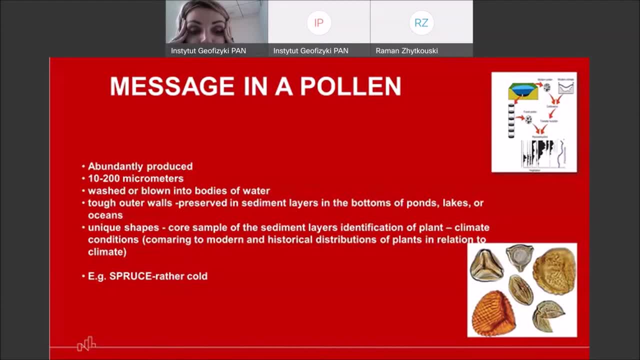 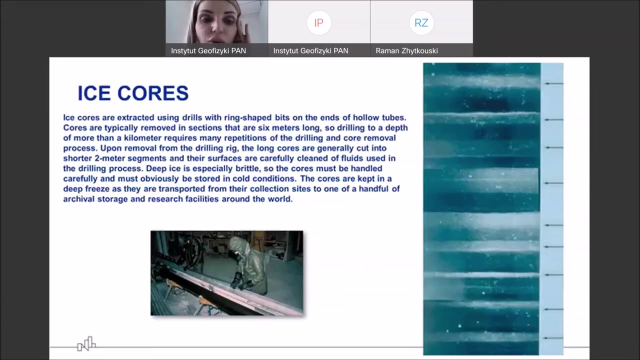 plants, we can determine what the temperature was like, what the weather conditions, climate conditions were like at any given time period when those pollen was produced. For example, if we find a lot of spruce pollen, it means that weather conditions were rather cold. Of course, the results are more exact normally- I mentioned that the Arctic, or 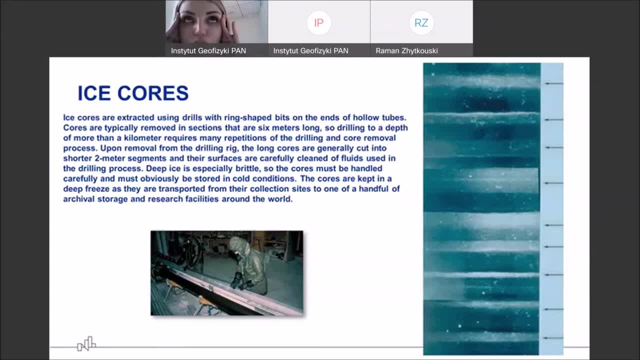 polar regions in general are a very rich source of proxies, And ice cores are what you can see here, which are extracted with drills from glaciers, but also from ice caps. ice sheets from Greenland and Antarctica give us a lot of information that are then stored and then stored in the soil. 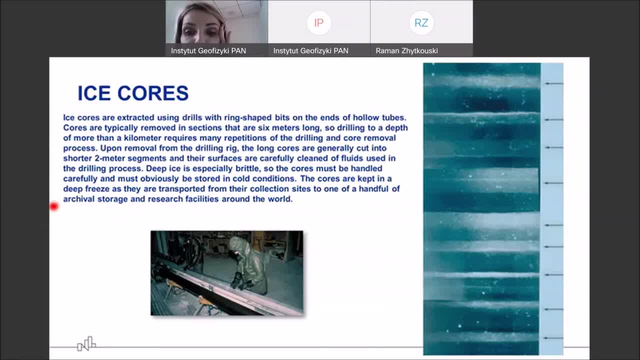 So probably they are the most comprehensive type of proxy record in the past climate. So we can perform physical chemical analysis of ice cores which provides us information on temperature, precipitation, atmospheric aerosols like volcanic ash sea the year without summer. 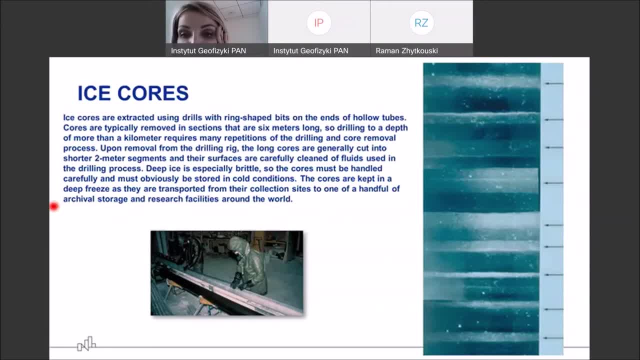 or even levels of solar activity at some point. So they can provide data and they can give us data on the annual activity of ice cores And we can actually measure the rate of precipitation. So we can measure the amount of precipitation that's recorded in the climate, with the soil. So that's something that we can do. 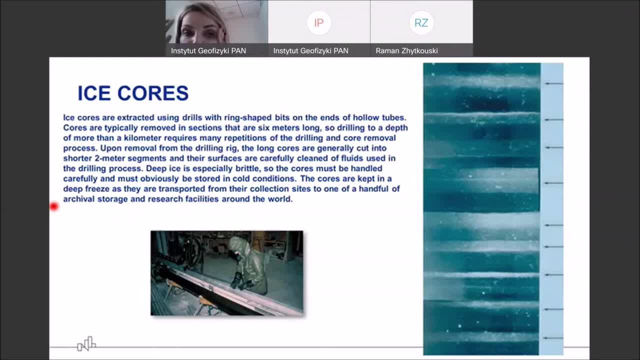 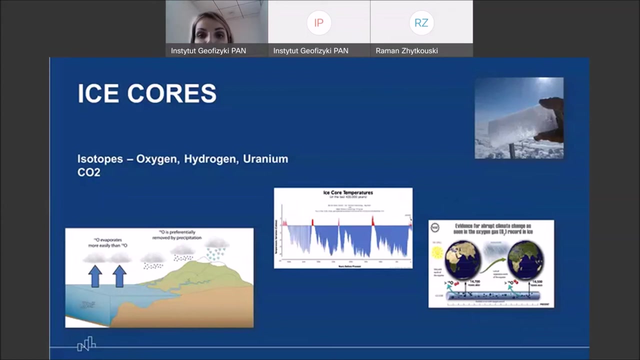 with a very fine resolution with high resolution. one year and, as some records spend periods of hundreds and thousands of years, so there are really really long time records. so what type of data is used and is drawn from ice cores so we can measure the gas composition, which is direct. so some gas was trapped in deep 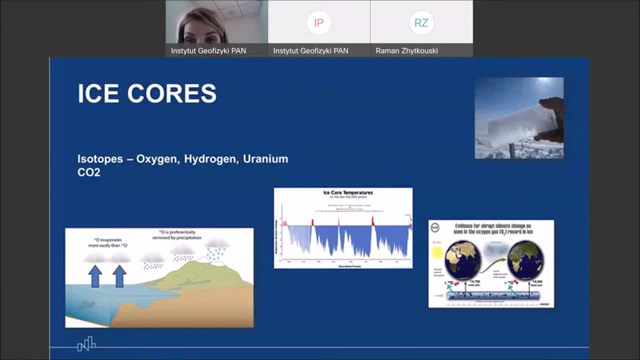 ice scores, tiny bubbles of ancient air, then we can extract and analyze using water and equipment. but this is a gas composition, if you have at. the temperature is not measured directly but most likely drawn from the isotopes as the decomposition of the water molecules which are released by melting the ice. So it's quite complicated about those molecules and 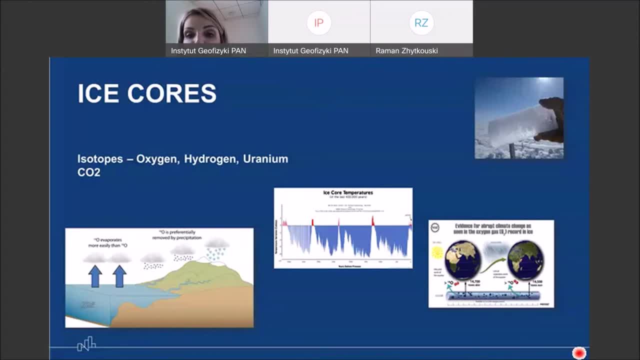 isotopes In general, we usually use oxygen hydrogen, especially oxygen, which has two stable isotopes: Oxygen 16,, so with eight protons, eight neutrons, and oxygen 18 with eight protons and 10 neutrons. So all these isotopes are stable, they do not undergo like a radioactive decay. so 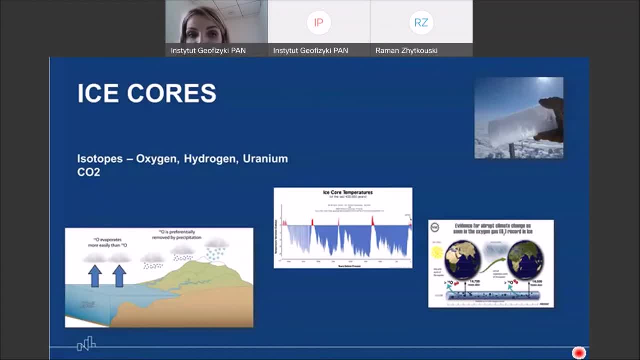 they are not like some radioactive isotopes, But also uranium, which is an radioactive, has been used to date some ice cores from Antarctica. So what we know from this image, for example, is that in general, the 18 oxygen is, we might say, a heavy oxygen and oxygen 16 is light oxygen, it's light. 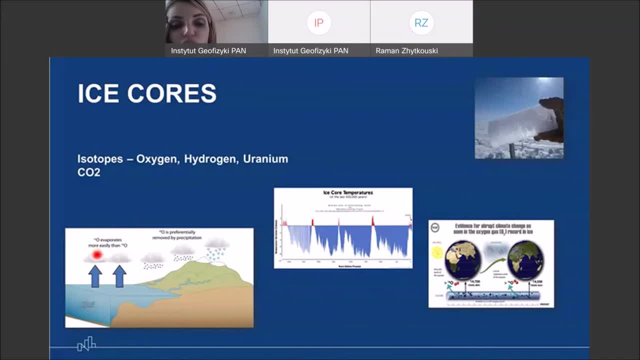 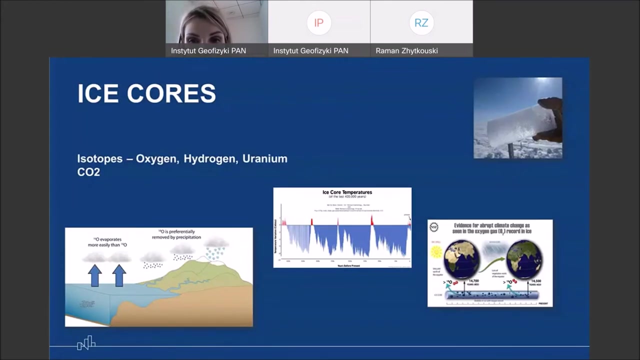 So if we find a lot of heavy oxygen in the archive, we can determine that it must have been really, really warm at some point so it evaporated, Because the heavy water evaporates not as easily as so-called light water. So if even this heavy water evaporated, it had to be really, really warm. 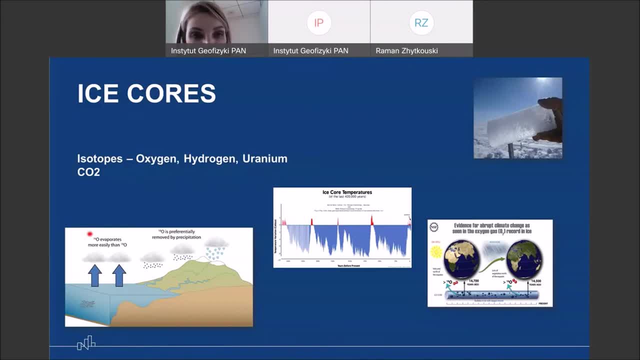 And these evaporation led to formation of clouds and then snow, and layers of snow create glaciers or ice sheets that we draw and drill ice cores from. So this is quite complicated, but it's. But in general, this is how, by comparing the content of different types of isotopes, 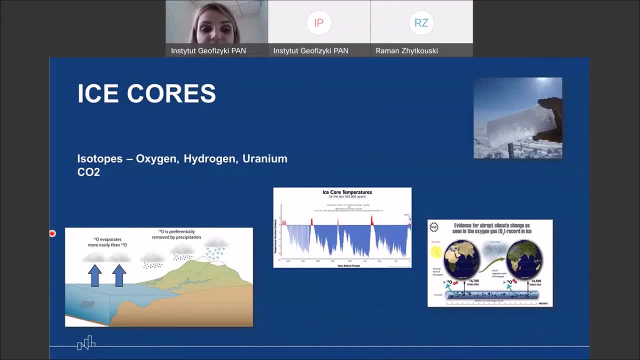 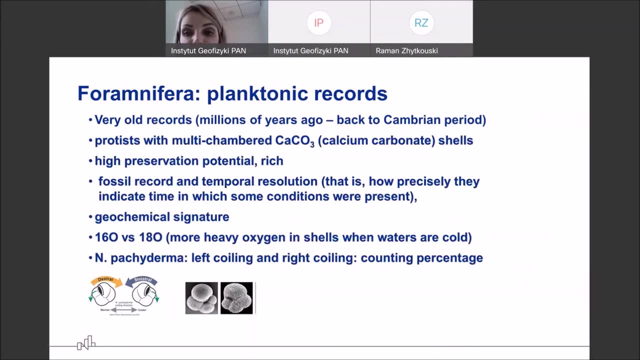 in ice cores, fellow climatologists can determine the temperature that was there at the time. Another type of proxy is a planktonic record, so-called foramnipera or forams. They are protists and they have a very tough multi-chambered calcium carbonate shells. 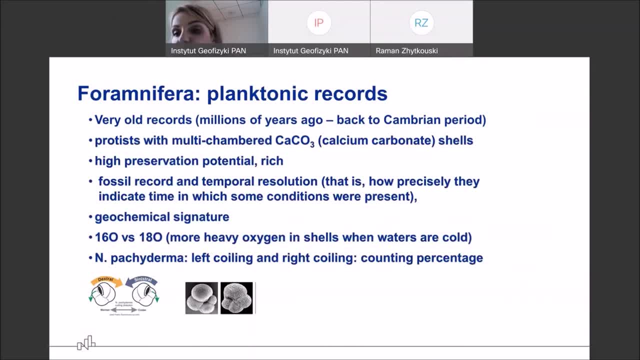 And they are very abundant as a fossil record, And so they are commonly used in reconstructing climate. They also live now, not only in the past. they live in upper zone of the open ocean, and they just incorporate geochemical content of water surrounding them. 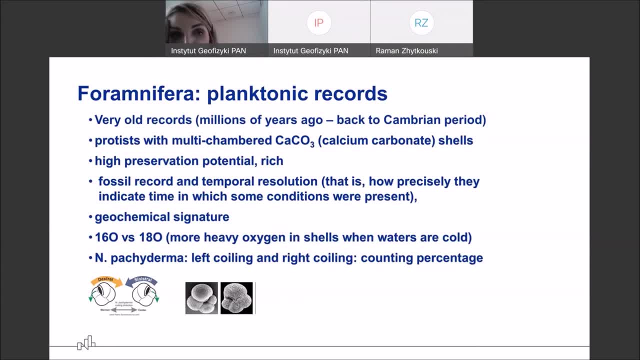 So what was their environment during their growth? So they absorb water that surrounds them and they preserve it. So, because they're very, very durable, they have those shells. they have a high preservation potential and it also provides very old records- Even millions of years go back to Cambrian period. 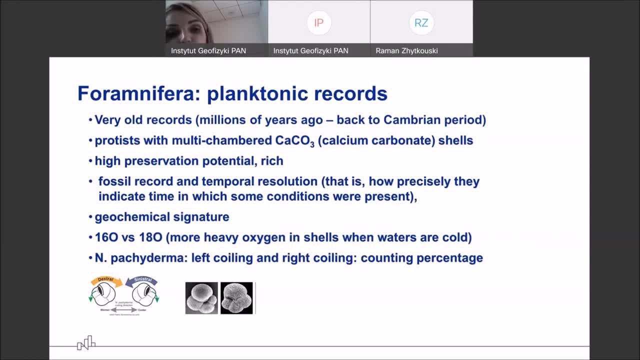 So… So they they're like a leftover, like a signature of those conditions. But there is another very interesting feature that they have. so they tend to form different types of shells depending on temperature, Left coiling and right calling. it is pretty funny, because When it's 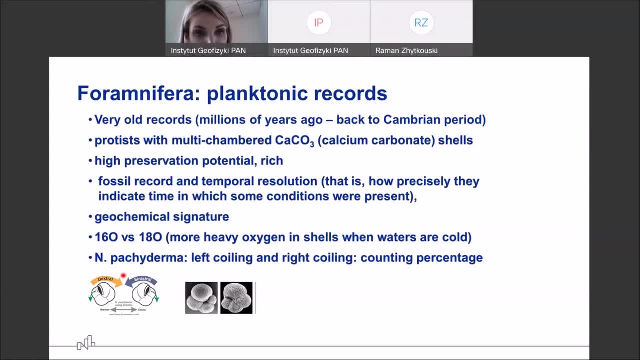 left. left calling it means that The temperature was lower, the weather conditions were colder, The climate was colder, but they tend to Create those right calling Shells when it's the other way around, so that when the climate is war. So if in some sample we find a lot of right oiling, 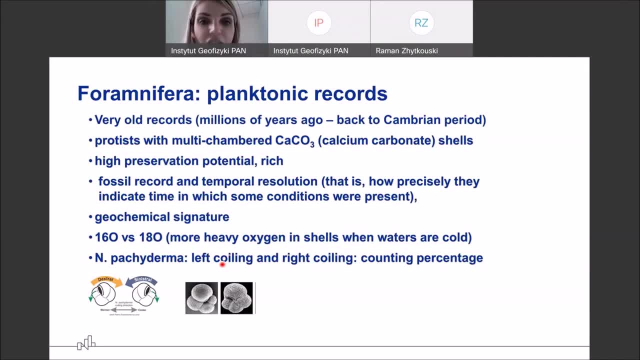 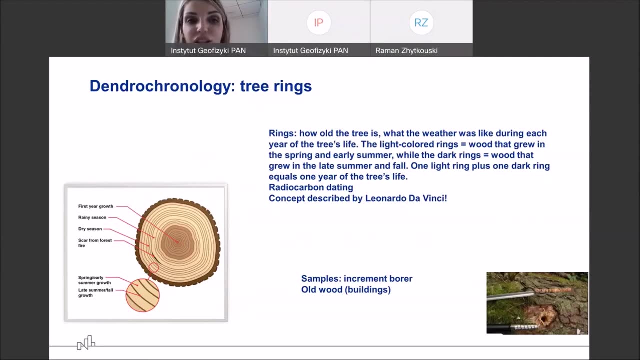 Forums such as Hederma, We discounted Percentage. Oh, there was a lot of right calling For us. it means it was warm at this at this time period. of course It's again. I'm just Presenting you a very simple form of that. It's more sophisticated in a measurement about the general radiators. 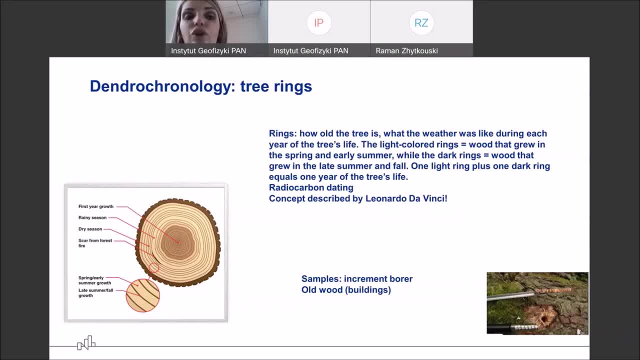 I won't really mention three rings Used to determine the age Of sample by counting three rings, but you can use three samples And so-called dental chronology for other purposes as well. There are archives, there are proxies themselves and Also you don't have to cut down the tree to study the three ring, I need only to collect the sample. it is possible whether this 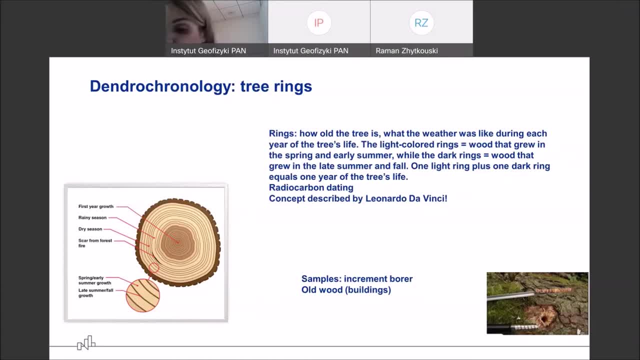 borer that you used to collect the sample without destroying the culture, and It extracts a strip of wood and and It goes all the way to the center of the tree and if you pull it out, Good to come to rings. but you can also observe the rings and 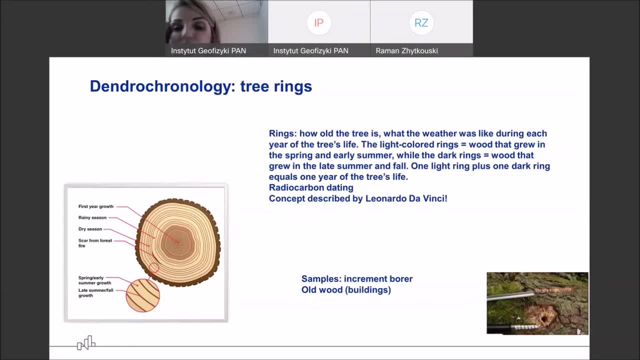 You. that means that You can observe how strong was the tree or how intense was the growth in any given year. so was it So? what were the conditions like? was it really dry with? Was it possible for the tree to grow, or was it really warm but also humid, so trees were growing abandoned. 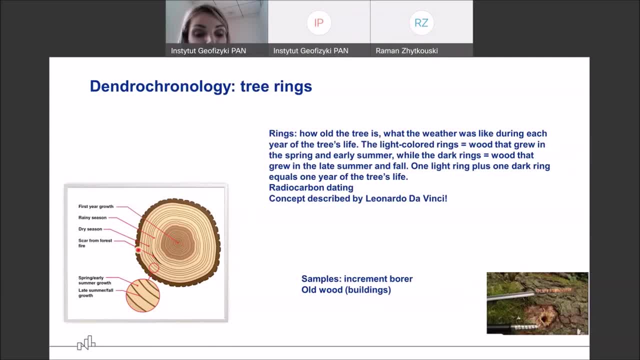 You can also find some scars left by fires, for example. But the problem with the endocrinology is that it doesn't provide a very long time span. so the oldest, really old endocrinological records Are for the south hemisphere. I are provided by some. 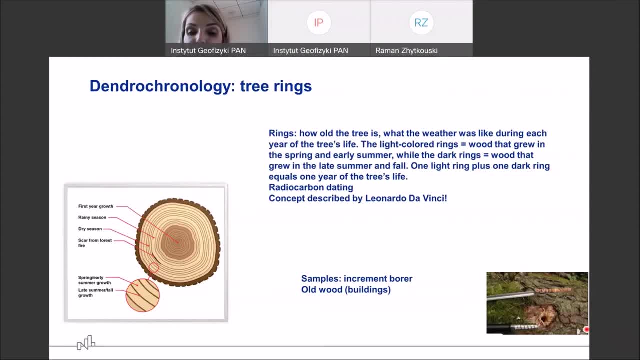 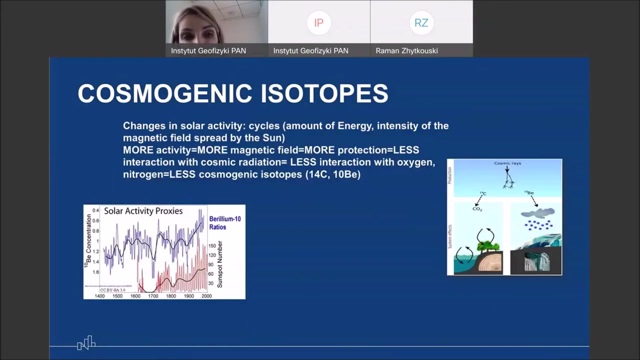 special trees, like, for example, Cyprus in Patagonia, and They date back to three hundred three thousand four thousand years. So they're old, but compared with forums that provide us with data from Million years ago, It's not such a long and wide time span Back to isotopes, another interesting fact that we can use. 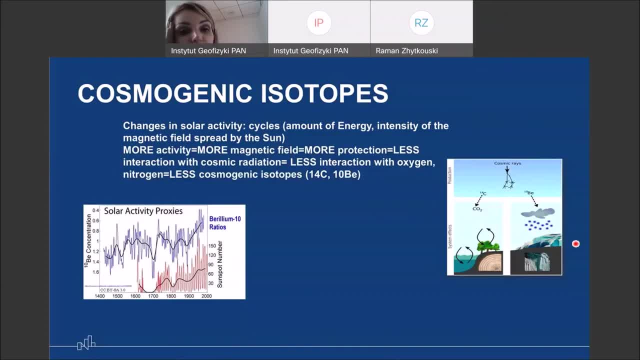 and that is used for follow by my ecological records and research and studies. We know and we observe that there are some changes in solar activity and we try to determine How this changes influence our climate. So changes in solar activity mean some situations in the amount of energy that is reaching the earth. 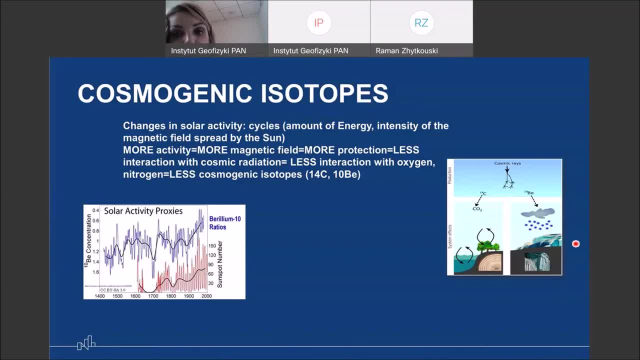 Also, There are some other consequences. There are also changes in intensity of so-called magnetic field, Because our star, the Sun, spreads magnetic field which is like a protective shield for the earth. It more or less protects years solar system from cosmic radiation. Cosmic radiation, which means accelerated charged particles. 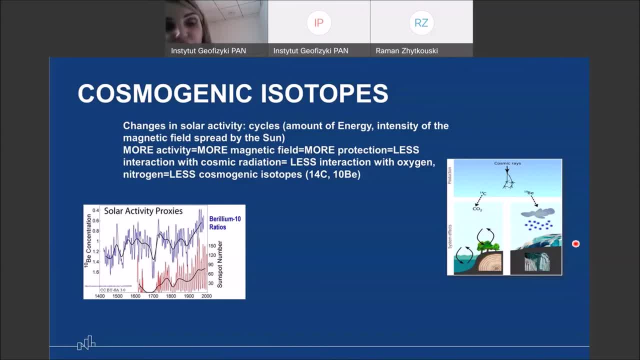 They are rushing through space, but, thanks to solar activity, We have a protective shield like a magnetic field, which is protecting us from this activity. so when this cosmic radiation, with this high energy accelerated cosmic molecule, collides with an Atomic nucleus located in a rock, soil or an atmosphere, 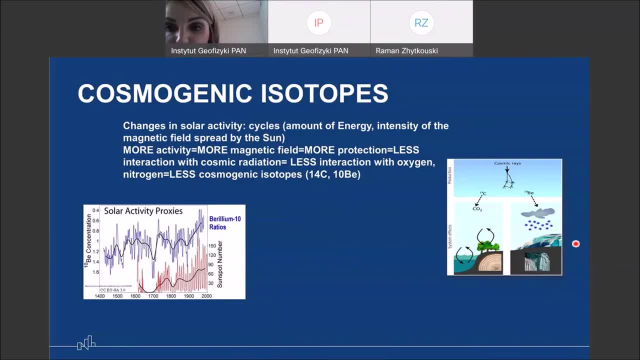 there is the undergo and nuclear transformation, and Some radioactive isotopes are formed that naturally do not exist on earth. For example, there is beryllium-10-beryllium isotope Produced in the atmosphere. also There's 14 carbon, so they normally are not there. 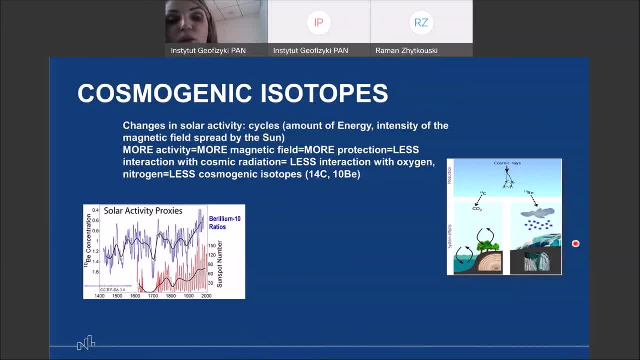 Naturally do not exist on earth. but so this is why we call them cosmic genic isotopes, because they are created because of this cosmic radiation. so if with this protective shield is Weak, that means there was not a lot of solar activity. that means a lot of. 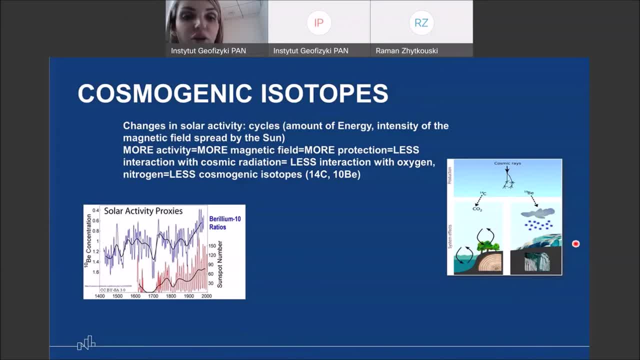 Particles collide with our atom in play and create a lot of cosmic. So the conclusion is: when there's There is a weak solar activity, not a lot of solar activity. we have a lot of Cosmogenic isotopes such as beryllium at that point. and the other way around, when the solar activity is really really intense and strong. 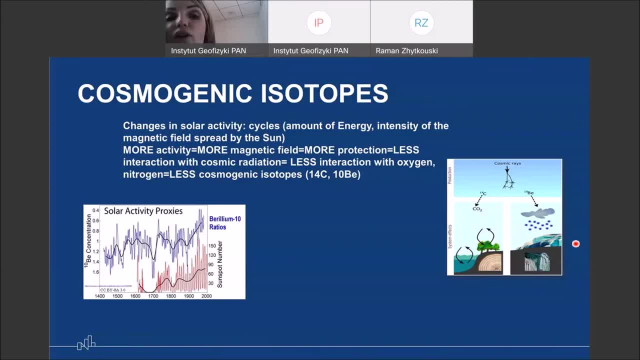 we have a strong magnetic protective shield and Not so many cosmic particles are able to collide, so we don't have a lot of cosmic genic isotopes. And then we are able to collect all this data from from from fallen from, from ice cores and so on and so on, and all this data combined help us recreate. 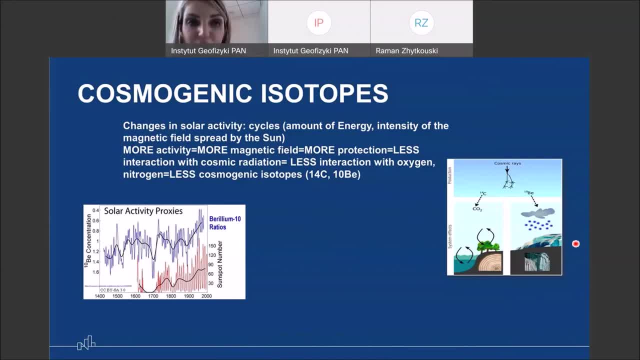 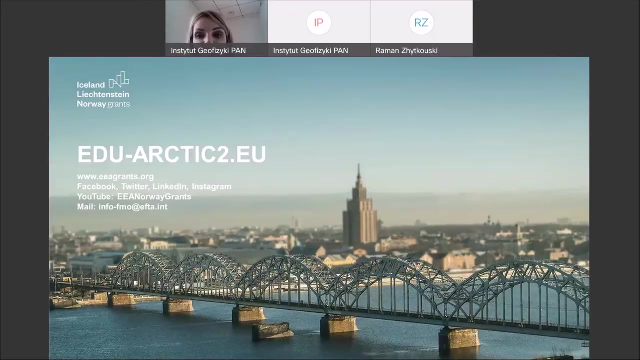 reconstruct the so-called polar climate and also draw conclusions. what were the conditions that caused warmer and colder periods? Was there some coincidence with increasing greenhouse gas amount in the atmosphere, or some other factors played the role? Thank you very much. This is all for today. 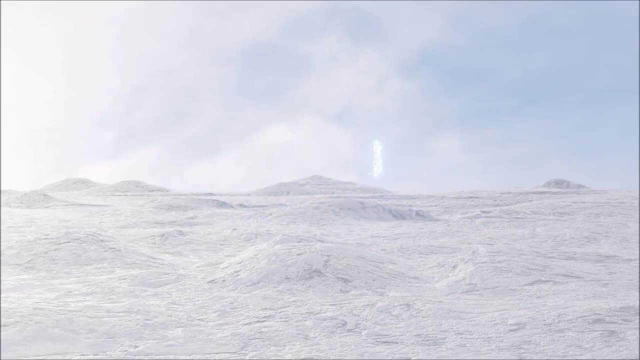 Watch other recordings from webinars on our YouTube channel: youtubecom- slash, edoarctic, edoarcticcom- From polar research to scientific passion. innovative nature education in Poland and Norway receives a grant of 240 000 euros, received from Iceland, Liechtenstein and Norway under EEA funds.